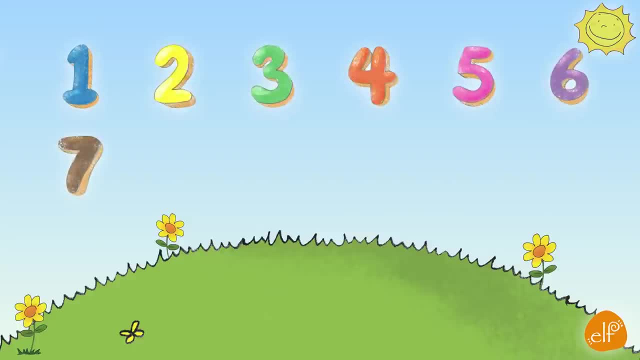 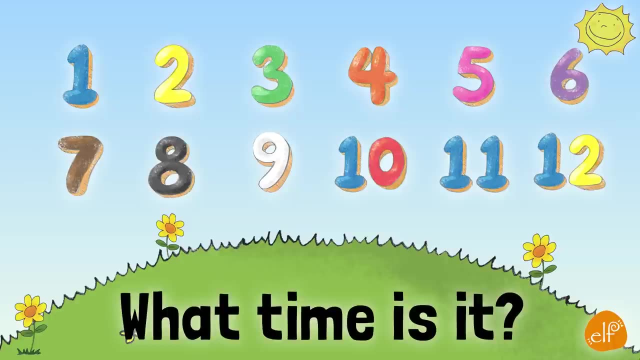 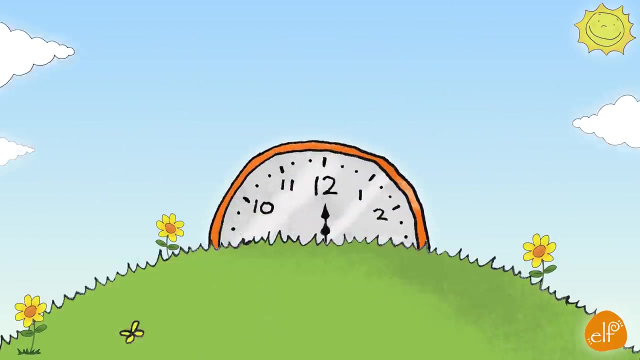 What time is it? 1,, 2,, 3,, 4,, 5,, 6,, 7,, 8,, 9,, 10,, 11,, 12. What time is it? Here we go. What time is it? 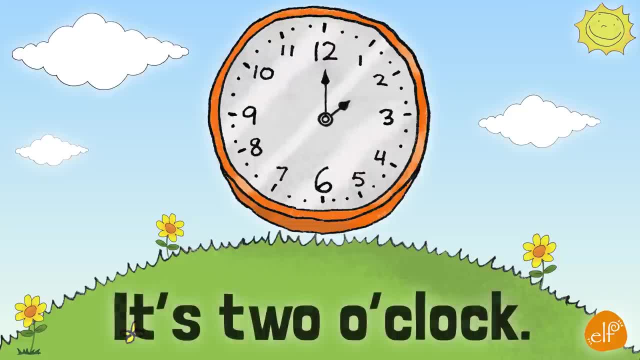 It's one o'clock. What time is it? It's two o'clock. What time is it? It's three o'clock. 1,, 2, 3. What time is it? It's four o'clock. What time is it? 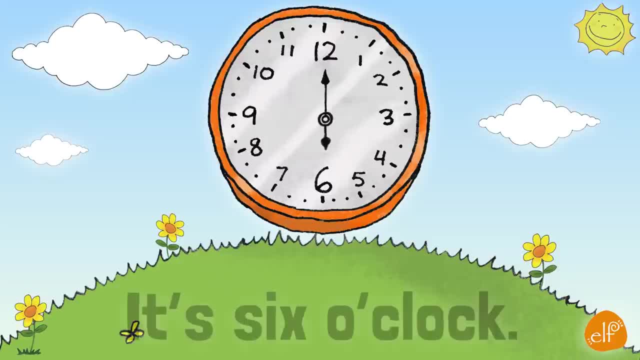 It's five o'clock. What time is it? It's six o'clock. Four, five, six. What time is it? It's seven o'clock. What time is it? It's eight o'clock. What time is it? It's nine o'clock. 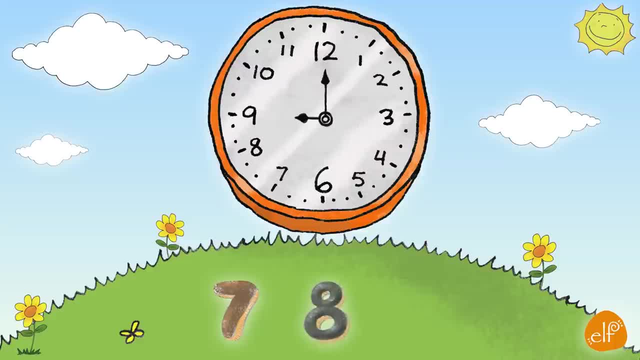 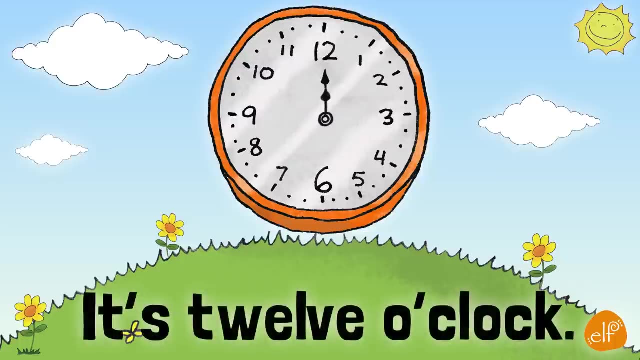 Seven, eight, nine. What time is it? It's ten o'clock. What time is it? It's eleven o'clock. What time is it? It's twelve o'clock. What time is it? It's twelve o'clock. It's twelve o'clock. 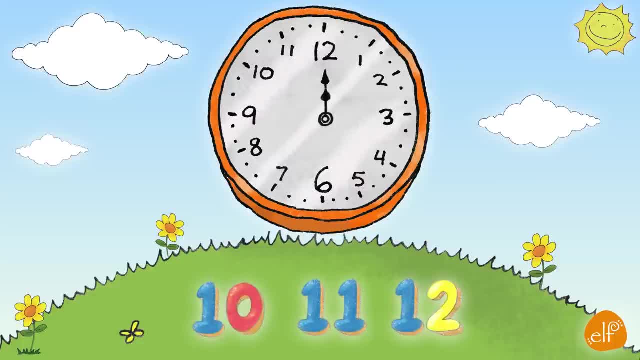 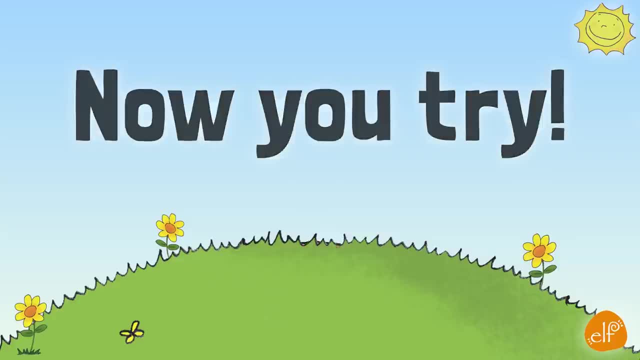 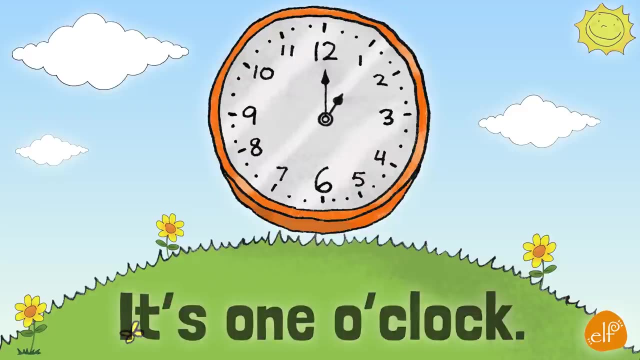